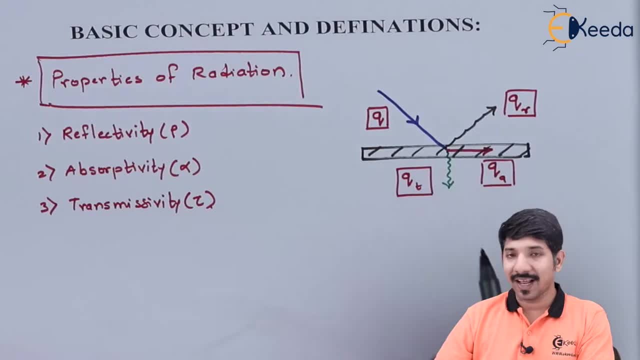 Let us say: Q of T is the amount of energy that is getting transmitted. Now, with this thing in our mind, what we can write down is: Q itself can be given as addition of these three Q of T. Now, this is nothing but the conservation of energy equation. 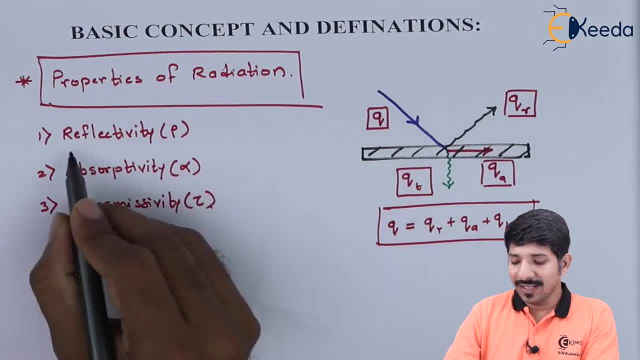 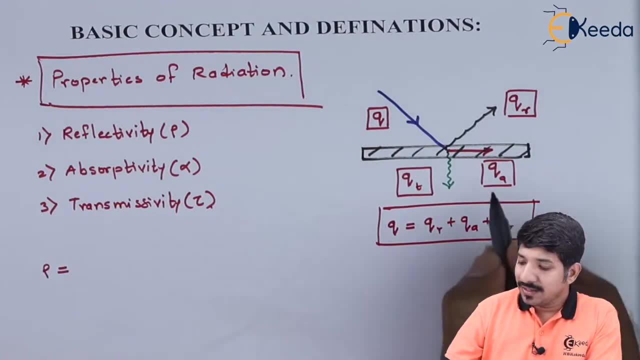 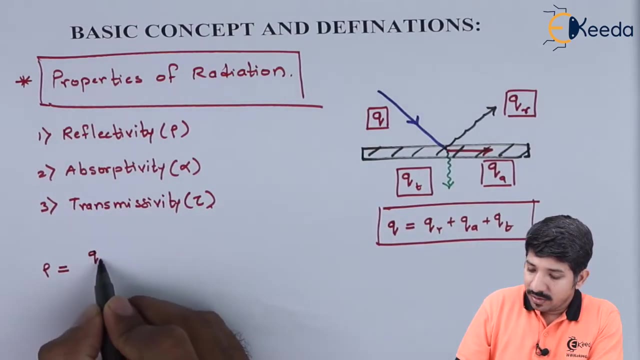 Then now let us look at each of this definition. Now, what is reflectivity? Now, reflectivity is nothing but the amount of energy that is reflected. So Q of R upon the amount of energy that is absorbed, Considered on a given body. 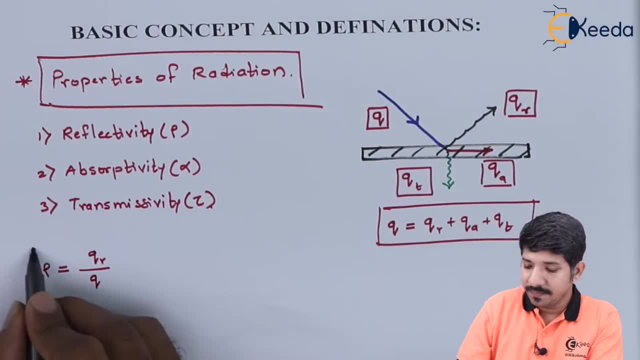 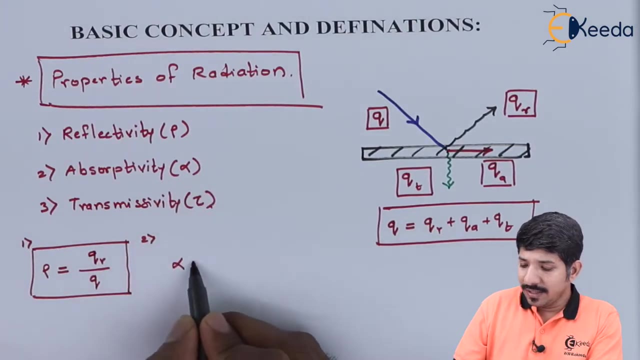 So it is Q of R upon Q. Similarly, the next one is the absorptivity. So what is that? Again the same. It is indicated by the alpha. It is nothing but the amount of energy that is absorbed by the given body upon the total amount of energy that is coming on to the body itself. 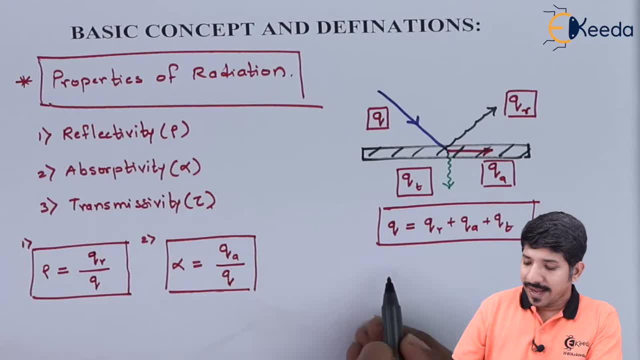 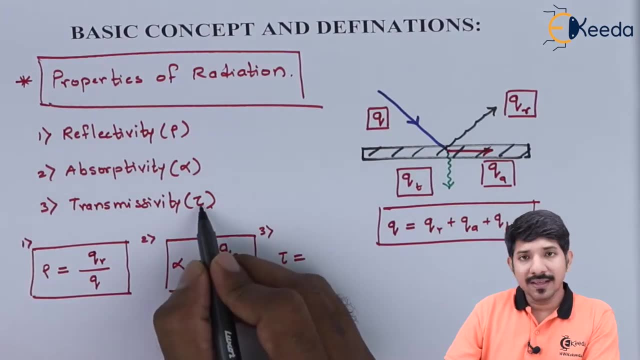 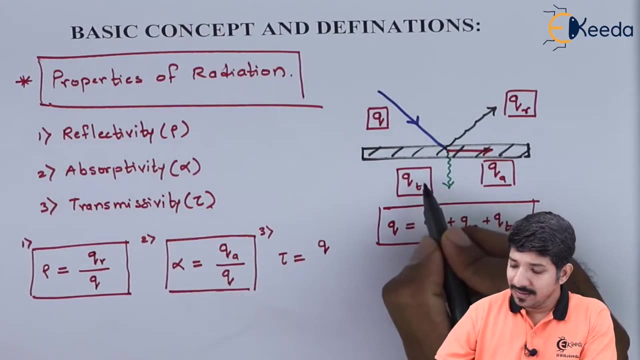 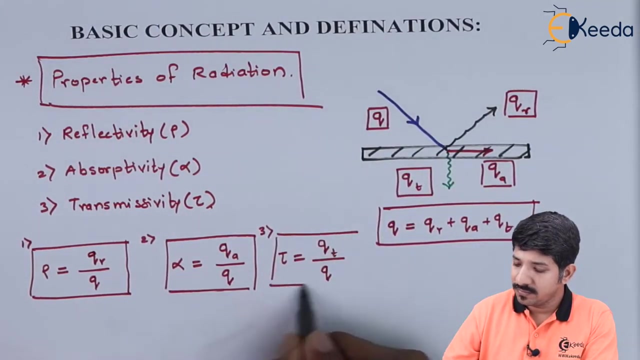 So that is the one, And then the third one is the transmissibility. It is indicated by this term tau. It is again given as the amount of energy that is getting transmitted. Q of T upon the total amount of energy. So these are the basic definitions of Q of T. 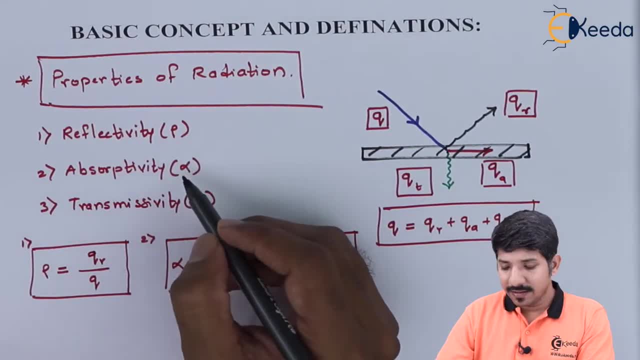 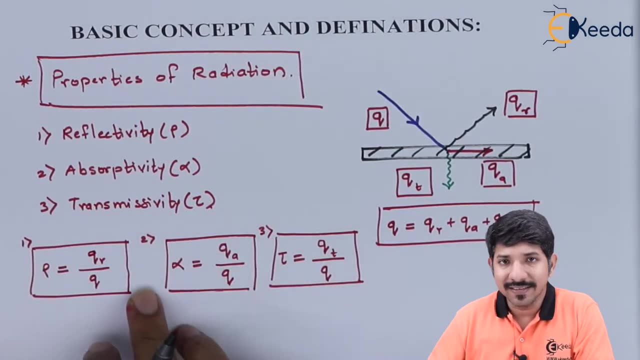 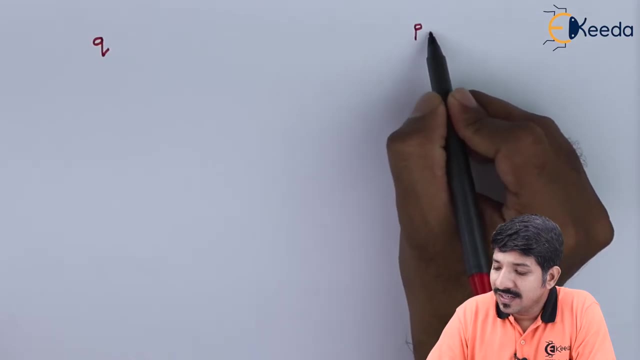 So these are the basic definitions of Q, of T reflectivity, then the absorptivity and then the transmissibility. So at the end of this description, what we can say, since if I add these three, equation means, if I want to write down what is the reflectivity plus the absorptivity plus the 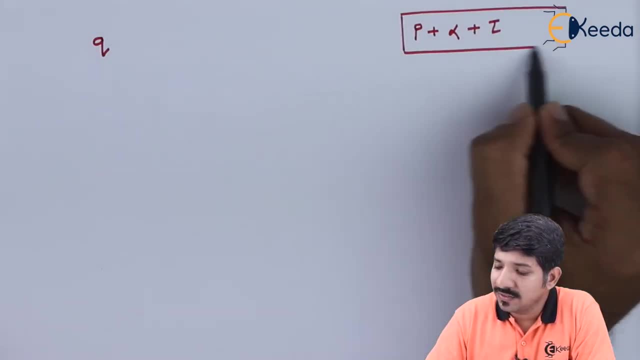 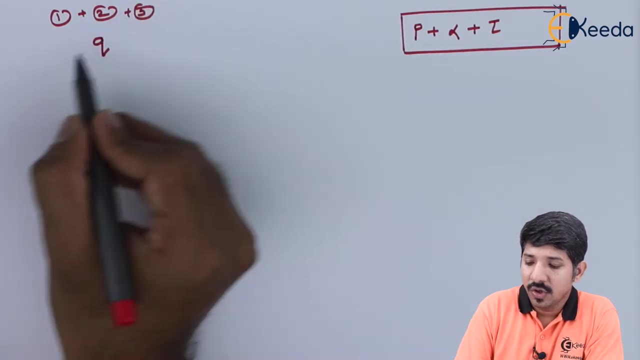 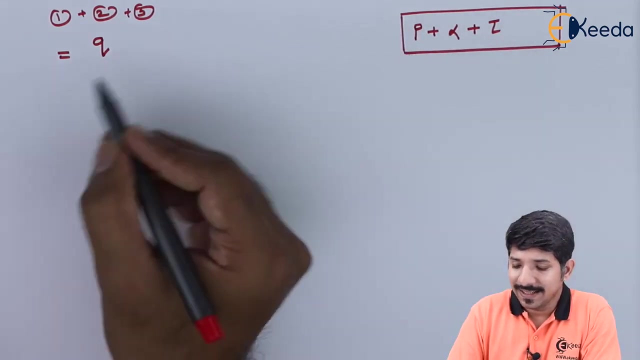 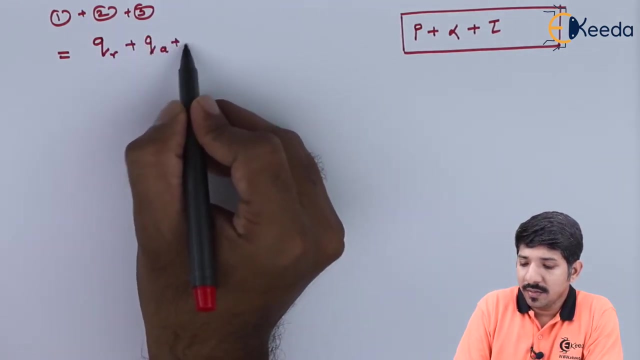 transmissibility. If I want to write down the equation for the same, I will have to add the three equations 1 plus 2 plus 3.. So what will that yield? The left hand side will be the same here, and then the right hand side will be QR plus QA. 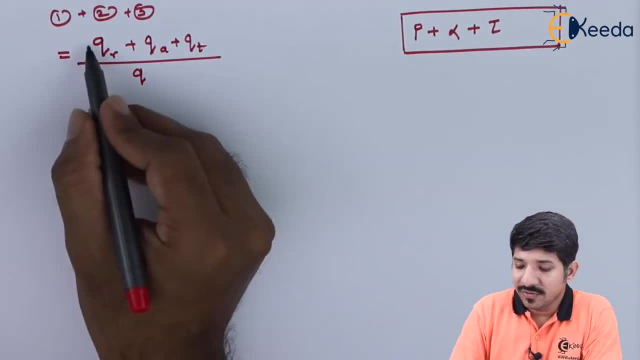 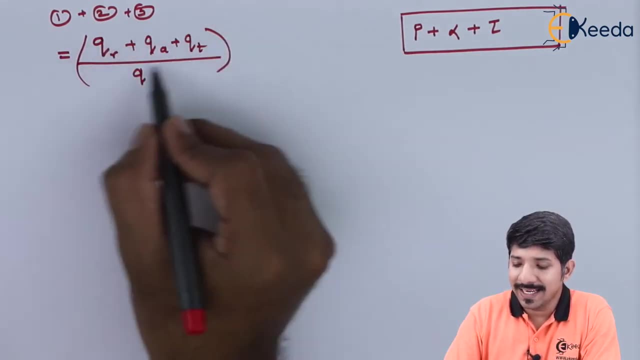 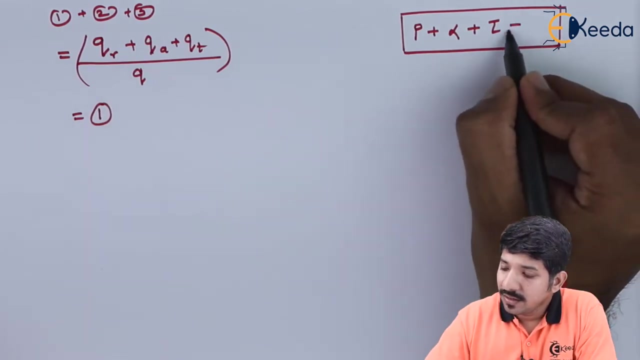 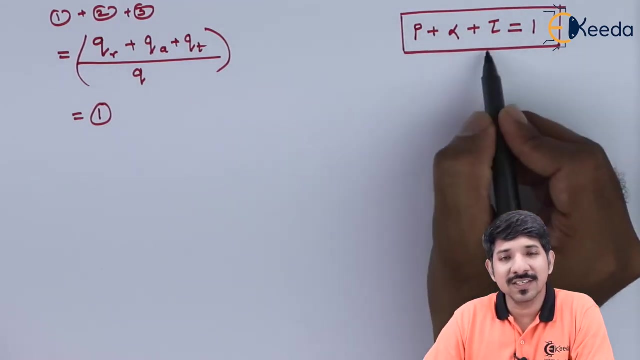 plus QT upon Q. But we have seen from the First law itself that this total Q is nothing but the addition of these three. So we can simply write down this as: 1 means what? The transmissibility plus the absorptivity plus the reflectivity, the addition of these. 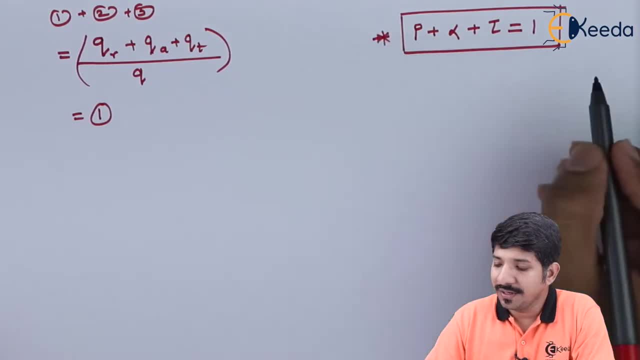 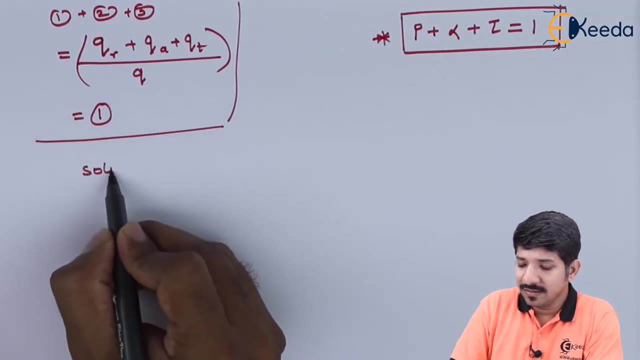 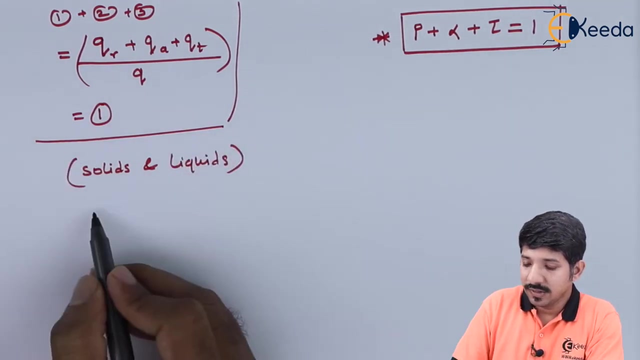 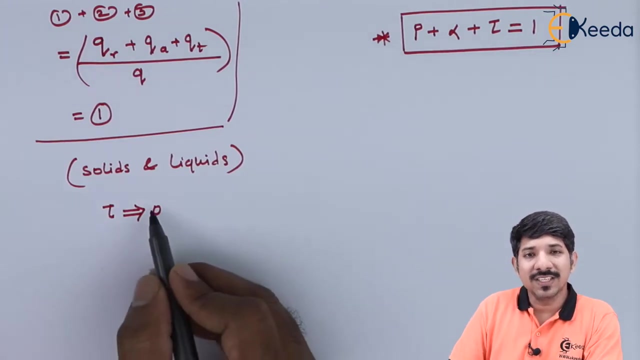 three should be unity. So this is one of the important point that we have found. Similarly, what we can say that in case of solid And liquids mostly the transmissibility is 0 means no amount of energy will get transmitted. Now again, this is not a hard and fast rule. 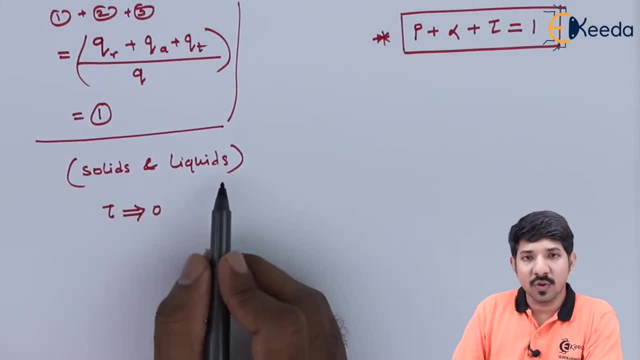 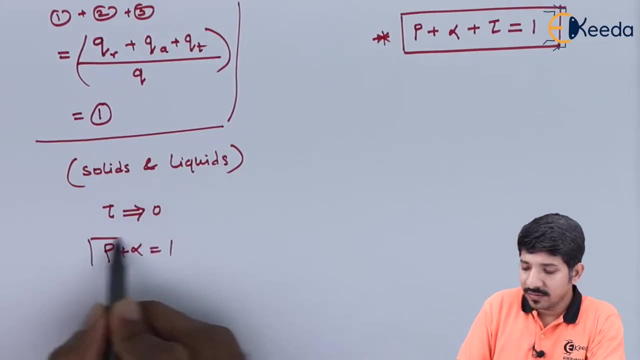 This is mostly for most of the solids and liquid, but not for the all. So in that case we can simply write down the equation as: rho plus alpha is equal to 1.. Okay, So if I know the reflectivity, I can find the absorptivity. 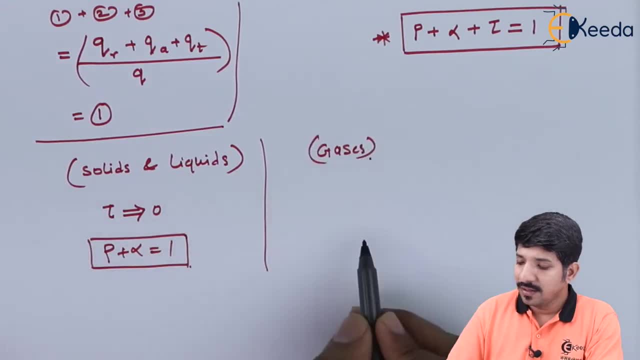 Similarly for the gases, I can say that there is no absorptivity, So alpha in this case tends to 0. So there is no energy that will get absorbed. So this way we can write down this as rho plus tau equal to 1.. 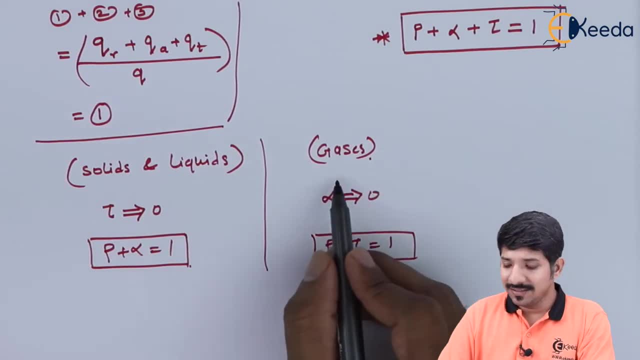 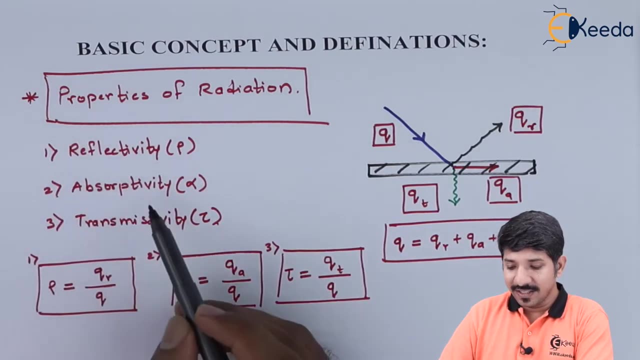 Again. Okay, So this is not hard and fast rule. These are mostly considered rule. So this is all about the property of radiation. We have seen that there are three properties: reflectivity, absorptivity and the transmissibility. 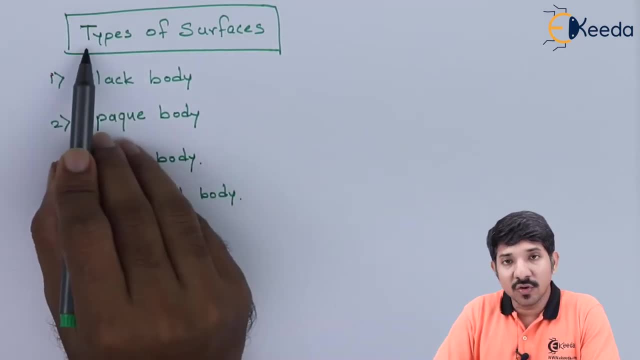 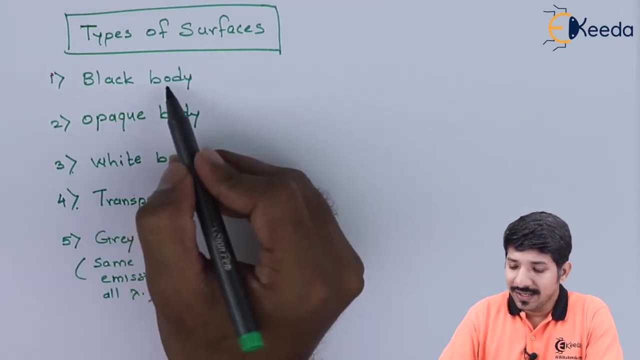 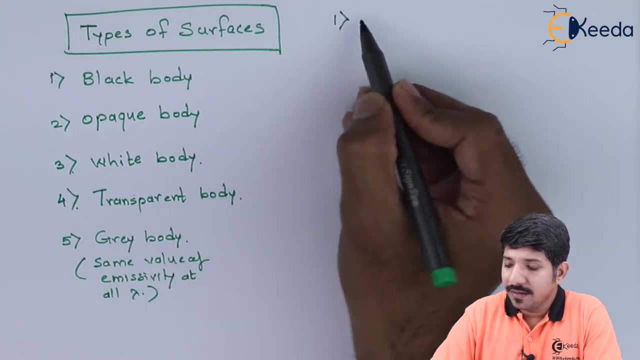 Now next is in the basic concept and definition. we are going to talk about the types of surfaces. There are, all in all, five types of surface that one need to study in the radiation. One is black body. Now, what is black body? So black body are those body where 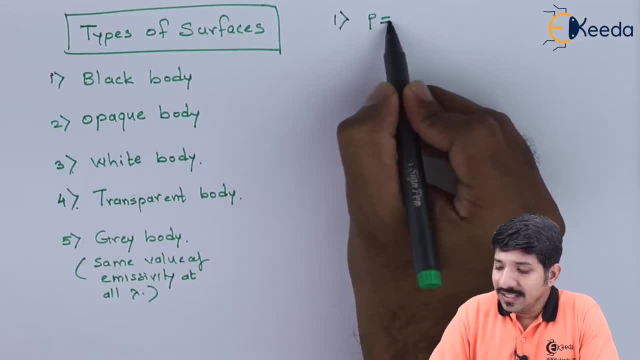 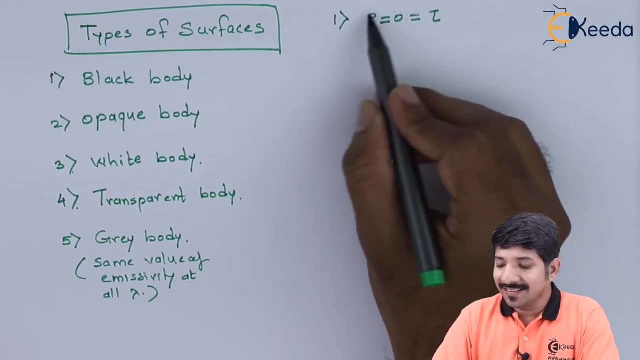 The reflectivity and the transmissibility is zero means the amount of energy that is coming on to this body. No amount of energy will get reflected or no amount of energy will get transmitted. So we can conclude that in this case, my alpha is always one. 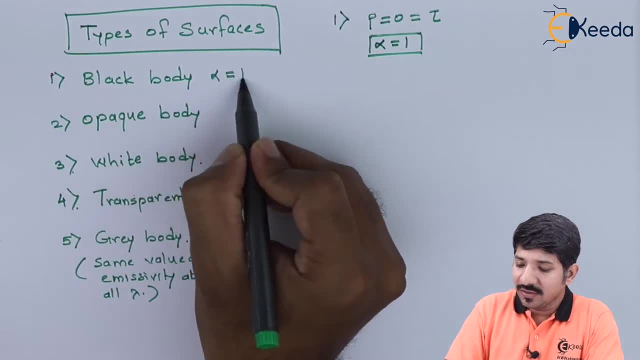 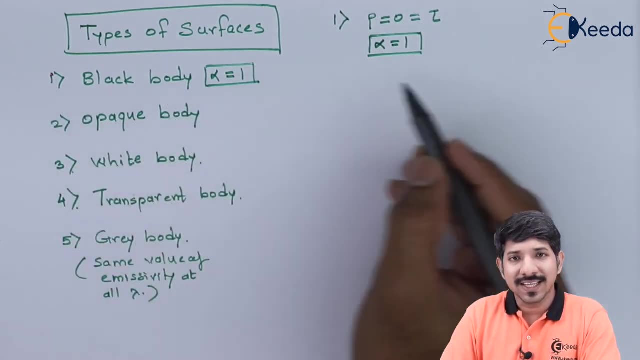 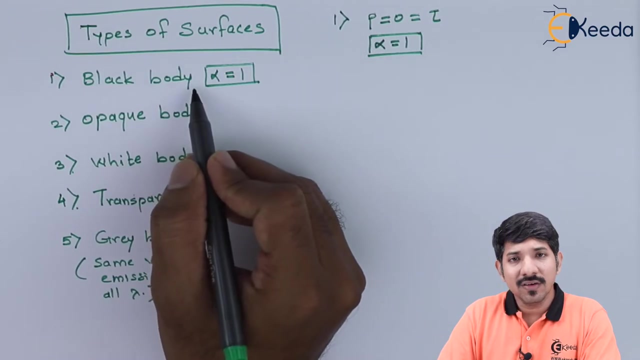 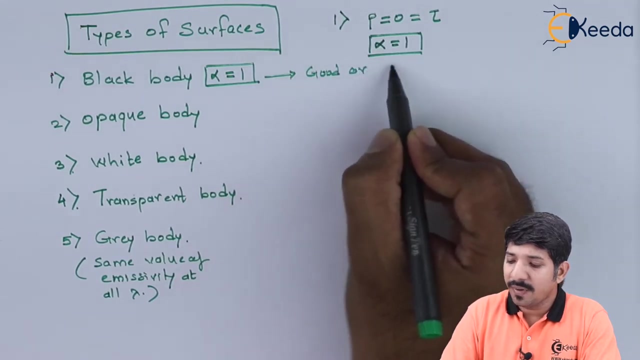 So in case of a black body, the value of alpha is always one. So these are the body where the amount of energy that is impinging on this body will entirely get absorbed. So black bodies are also considered a good emitter. So they are good or ideal, or perfect emitter. 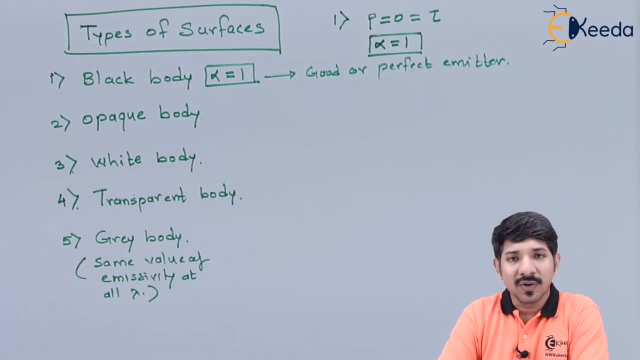 Again, this black body. there is nothing as such black body. Okay, So this is basically a hypothetical scenario or the hypothetical concept that they have invented for the ease of analysis in case of radiation, But in practice there are some cases which we can equate with that of the black body. 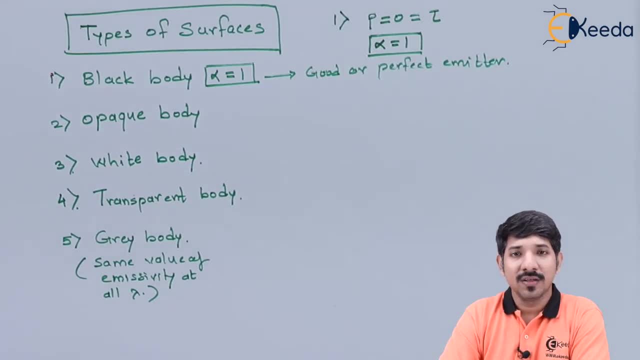 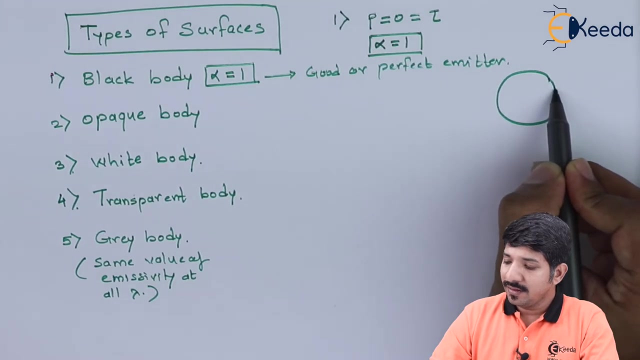 such as a black color lamp or the body entirely covered with the milk. These sort of bodies can be considered as a black body. One more example is- this is an experimental example that they have done Okay. So they have made a small section like this: 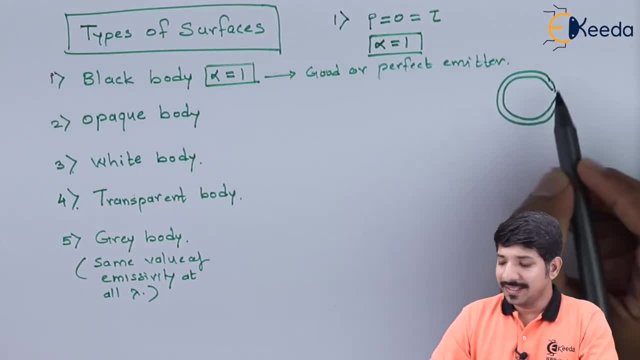 Now this is made of very high thermal conductivity. let's say, Then, the amount of energy that is coming on to this body- Now, this is entirely this is they call as a equivalent to the black body- Then the energy will get trapped inside. 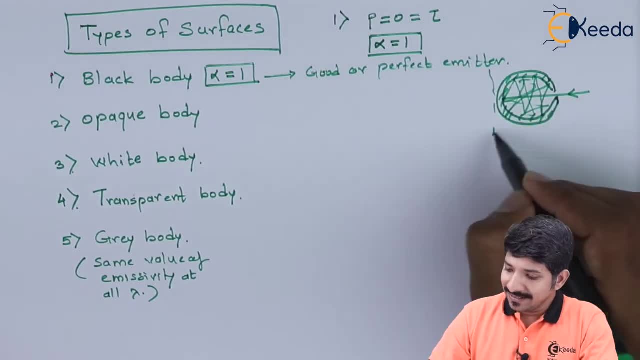 So there is no energy that will come outside. Okay, So in that case this body can be equated with that of the black body, where the energy can only enter and the entire energy that is coming onto this body is getting absorbed. No energy getting reflected, neither any energy is getting transmitted. 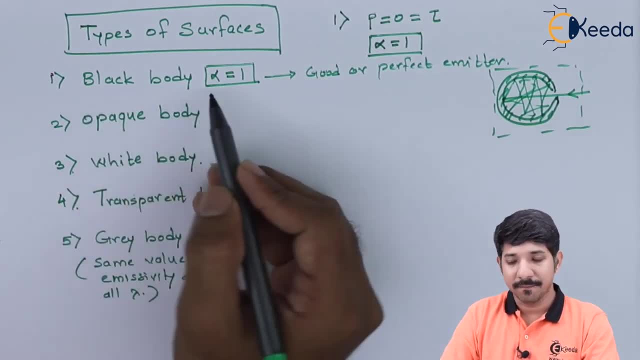 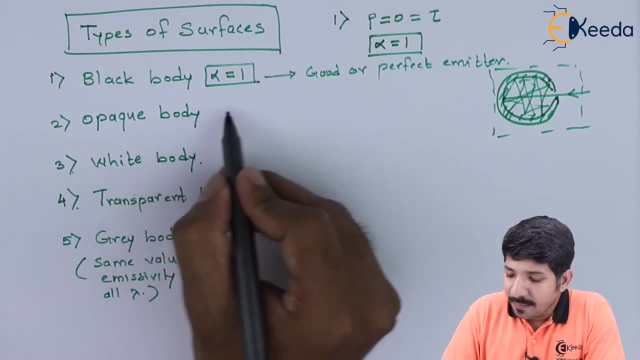 So this sort of body can be equivalent to that of the black body. Now, next one is the opaque body. Now, what is the opaque body? Now, in case of an opaque body, In case of an opaque body, There is no transmissibility. 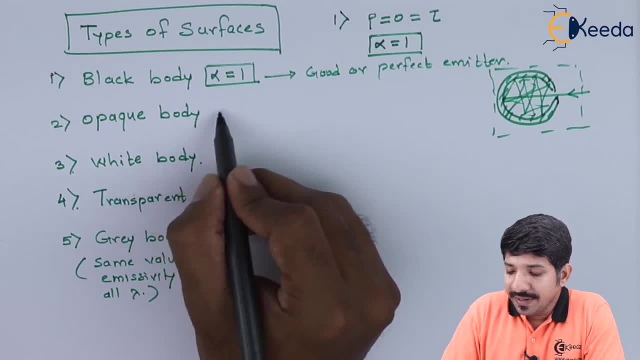 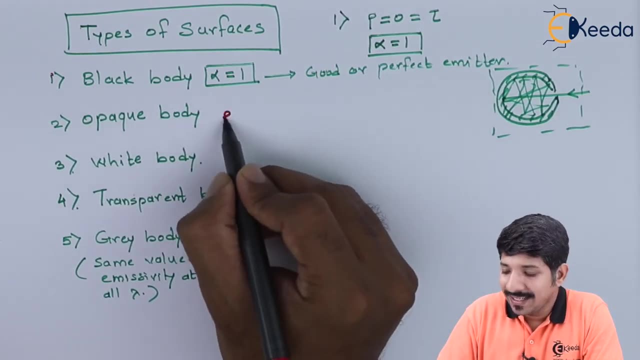 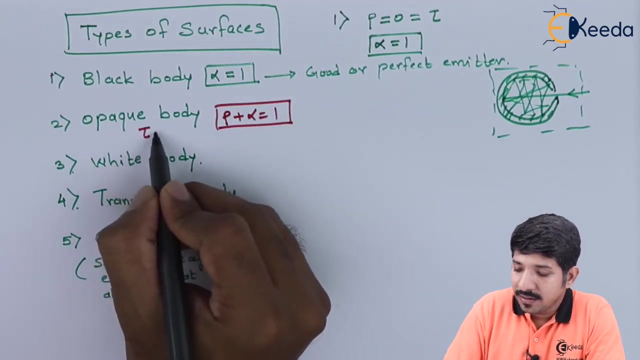 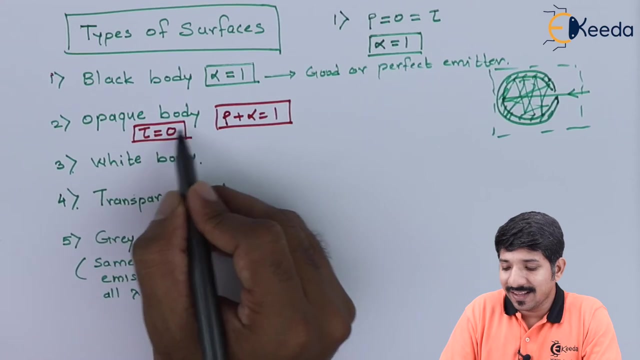 So the amount of energy that is impingent on this kind of a body will entirely get either reflected or absorbed. So I can write this as rho plus alpha is equal to 1 or tau is equal to 0. So, no matter of what, there is no energy that will get transmitted in this case. 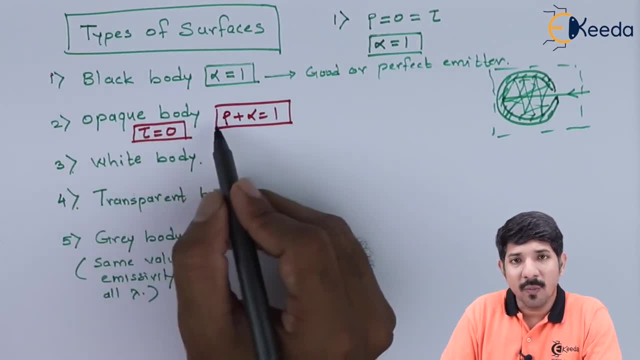 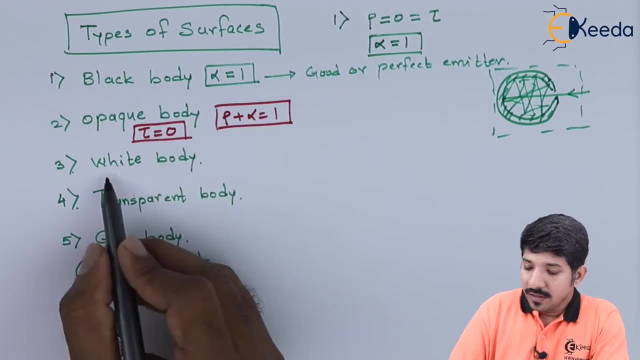 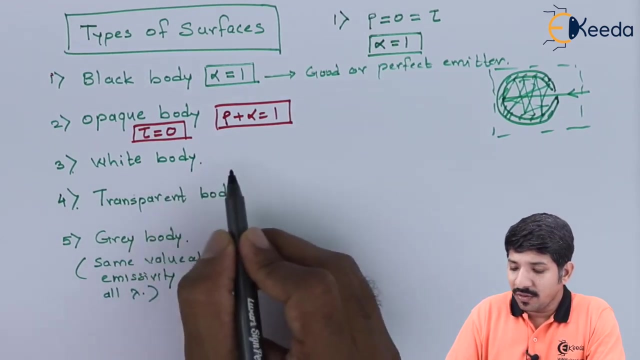 So most of the solids are opaque. Okay, So this can be considered as the opaque body, because in most of the scenario there is no energy that will get transmitted through the solids. Then we can talk about the white body. So white bodies are nothing but those bodies where the amount, the entire amount of energy 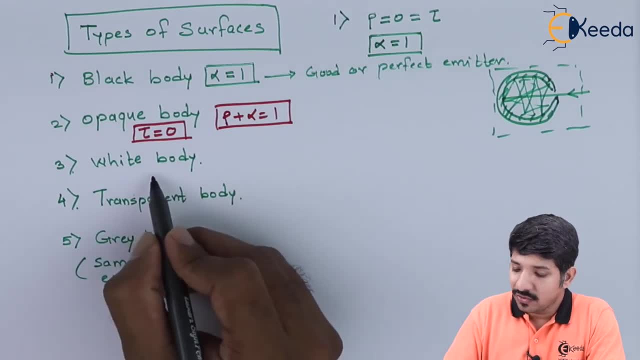 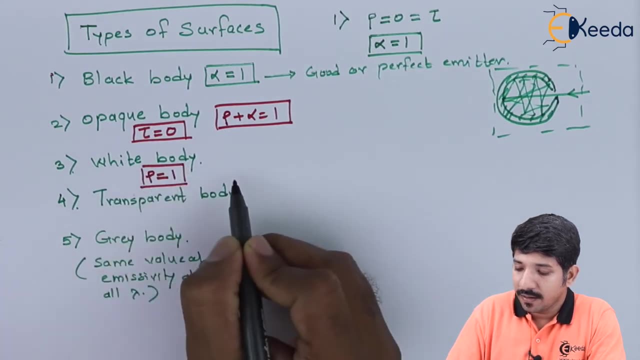 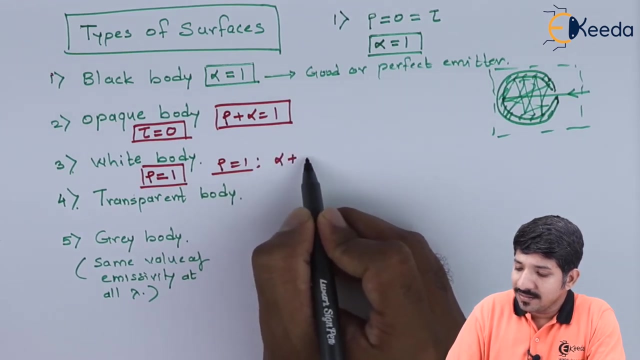 that is impingent on this body will get reflected, So rho can be considered as 1.. Means no amount of energy. Okay, So rho is getting either transmitted, So this is either. this is 1.. So alpha plus tau is 0. 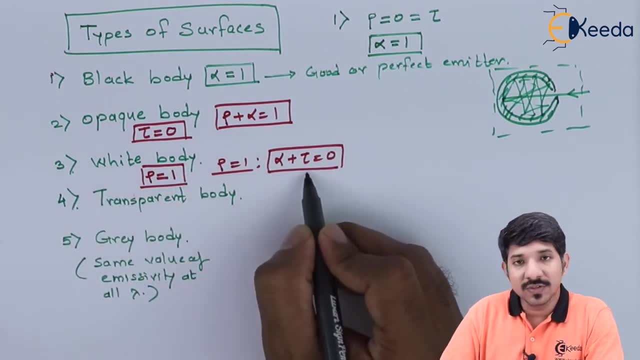 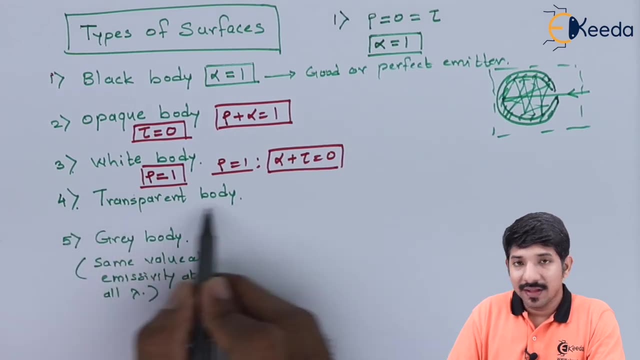 In case of a white body, the absorptivity and then the transmissivity is 0. Then, finally, the fourth one is the transparent body. Now, what is transparent body? Obviously, The entire amount of energy is getting transmitted, So tau is 1 in this case. 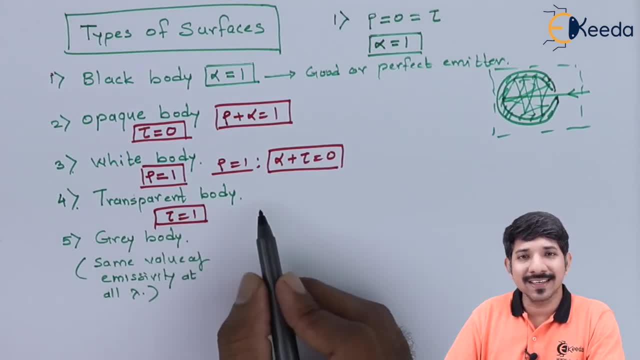 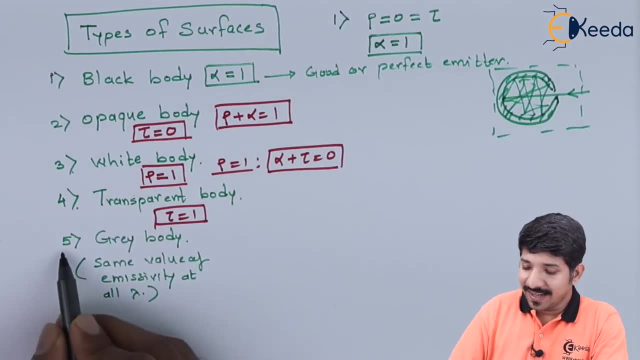 So no body or no energy is getting absorbed, or neither energy getting reflected in this case. So that kind of body is the transparent body And finally, the important one is a gray body. Now, what is gray body? So gray bodies are nothing but those bodies where the emissivity and the absorptivity 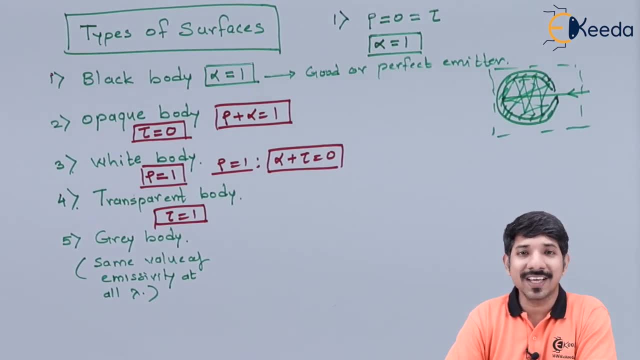 is almost same, Continuous. So conditionally, the temperature is kept constant for the two bodies. or we can also explain this as the same value of the emissivity at all the wavelength. So no matter what is the wavelength of a impinging radiation, the value of emissivity will always. 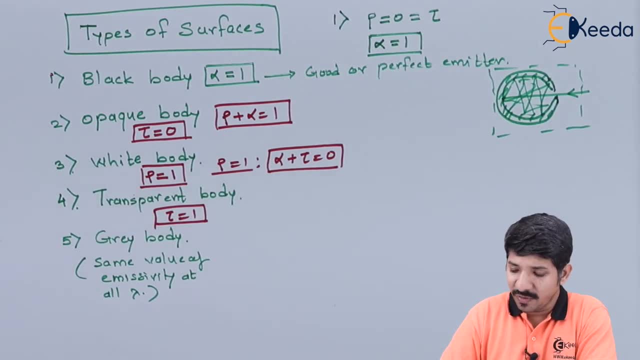 be same in case of a gray bodies. The best example of gray bodies are most of the metals, so they can consider as a ideal example of a gray body. Now, in this topic we talked about the property of radiation and the types of body. 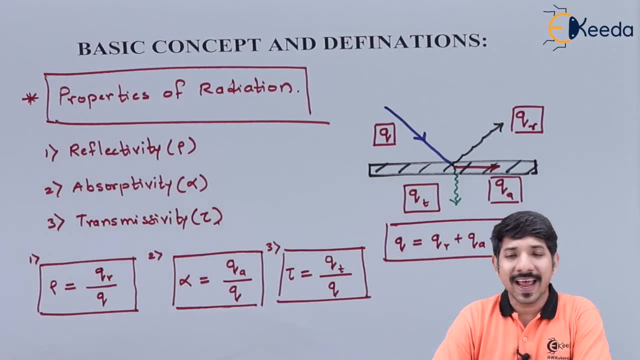 Obviously, they depend on the nature of radiation and then the type or the finishes of the surface of a given body. Based on these two parameters itself, we will have to do our analysis in case of a radiation. That is it in this topic.